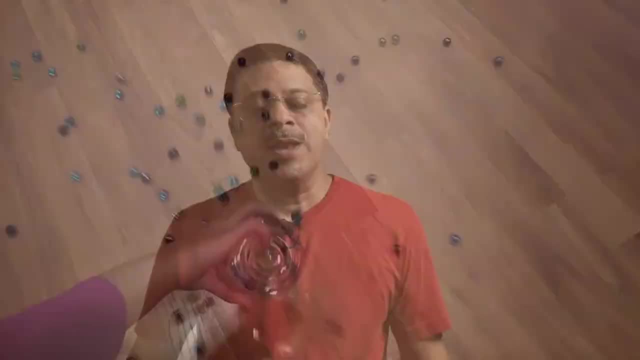 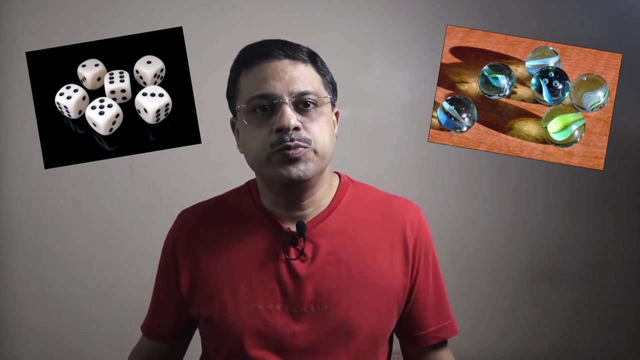 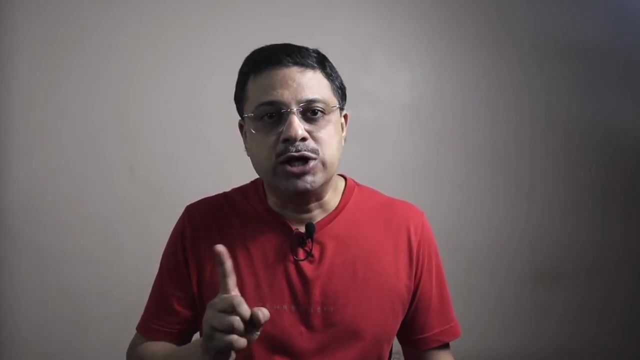 instantly think of rolling dice and or coloured marble. Real life is not about rolling dice or, for that matter, studying marbles of any colour, be it red, green or blue. Real life is about real problems and real problems require real solutions, not dice and marbles. Uh-huh, marble and dice is definitely. 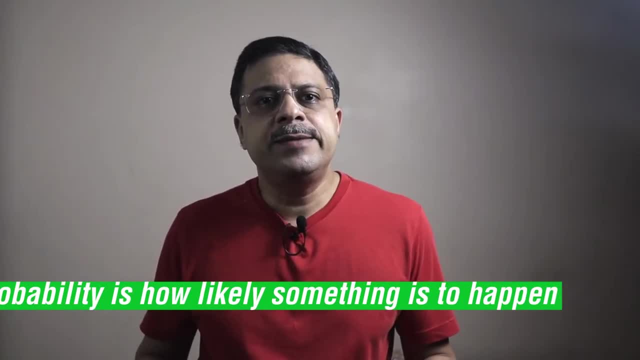 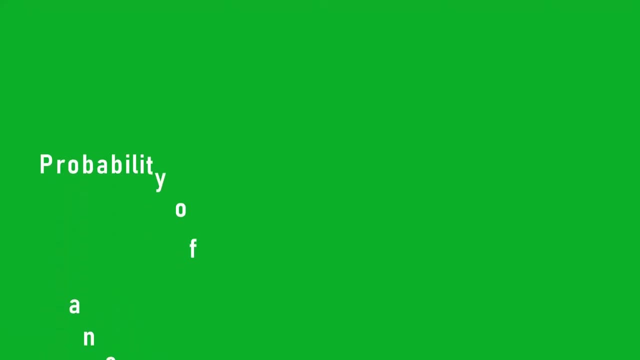 one thing that we are not doing in this video. Probability is simply how likely something is to happen. Whenever we are unsure about the outcome of a problem, we are likely to think of it as a probability of an event. We can talk about the probabilities of certain outcomes Mathematically. 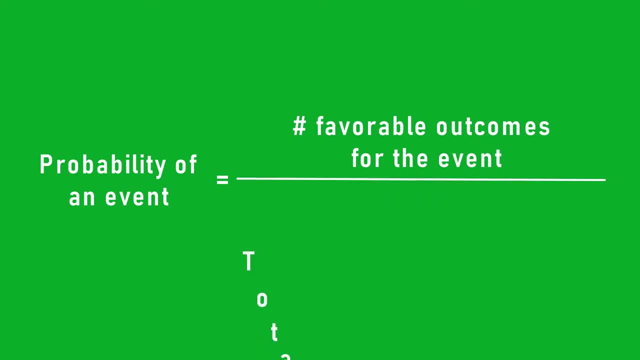 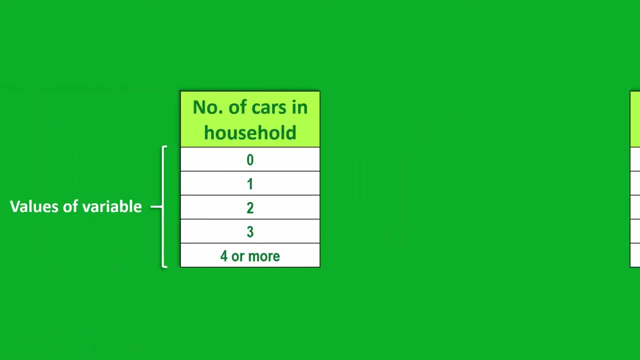 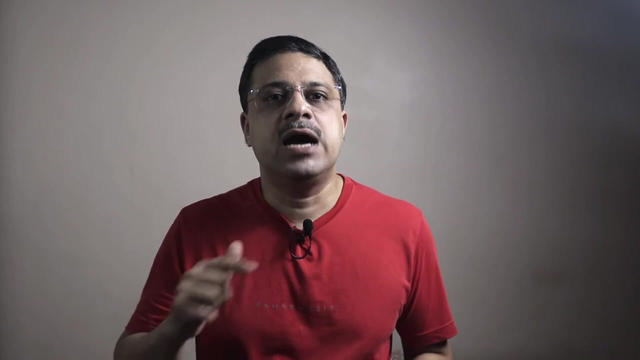 put, probability of an event is the count of favourable outcomes for an event divided by the total number of favourable outcomes, And distribution is the possible values a variable can take and how frequently these values occur. Let's see what is happening with this car manufacturer. 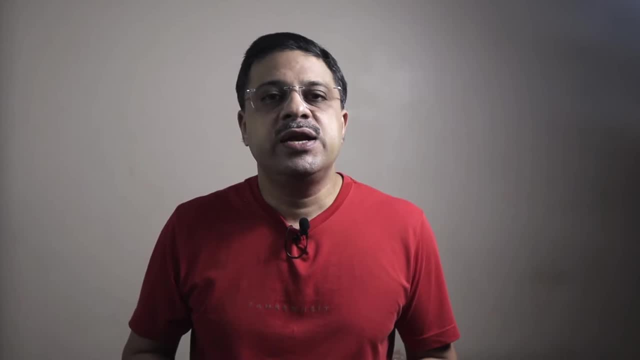 A car manufacturer, Tomota cars, conducted a study in a region of a state. 300 households were chosen in such a way that they represented all the households in that state. The households were asked to state the number of cars owned by them. Following is the data: 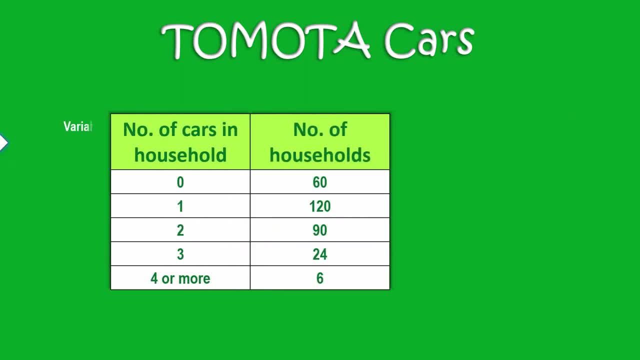 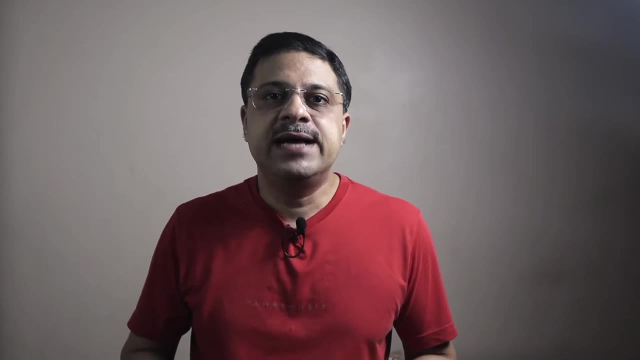 represented in this table. The variable here is the number of cars owned by a household. The values taken by the variable range from zero cars to more than four cars. Number of households represent the frequency for each value of the variable Going further if these households are. 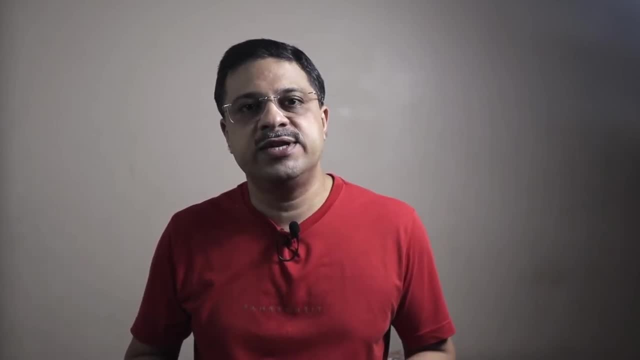 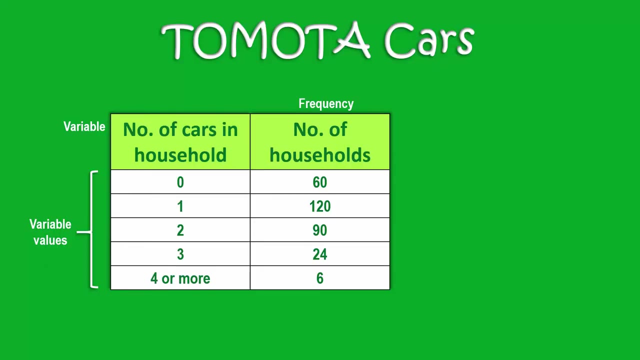 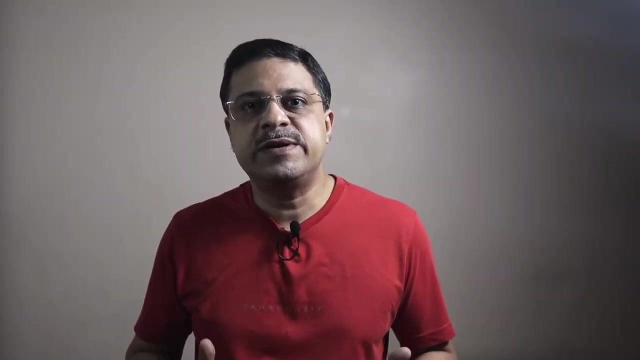 represented the ownership of cars in all the households in a state, then we can safely say that the likelihood of the ownership of cars in that state is represented by the probability column. like so: The probability is calculated by dividing the number of households owning a specific number. 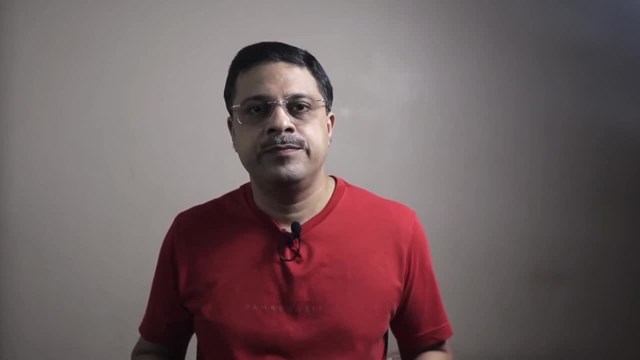 of cars by the total number of households, that is 300.. Obviously, it's physically difficult to interview each of these several million households in the state, So we use probability. The probability column for the various values in the table depicts the probability distribution. 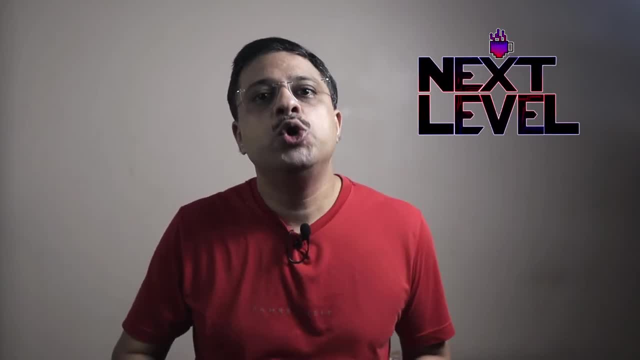 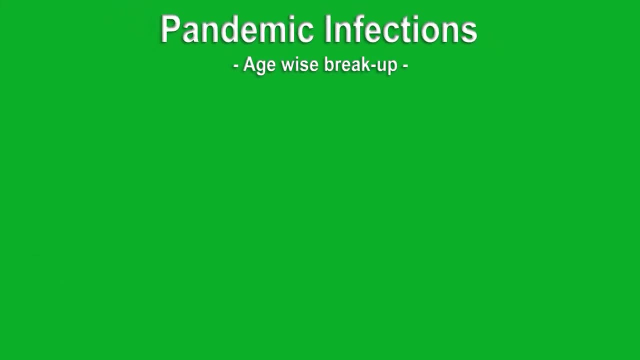 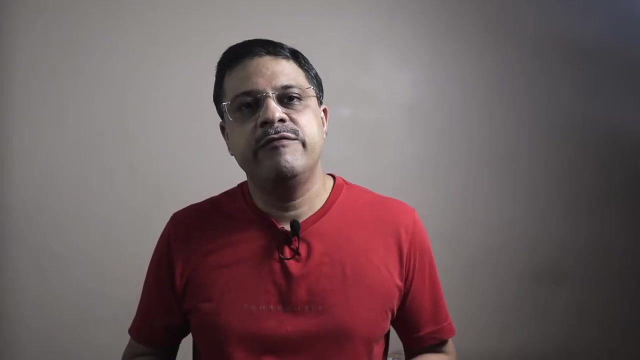 Alright, so if this was not daunting enough for you, let's go to the next level of the game. The following table illustrates the number of coronavirus infections by age group reported in a state on April 26, 2020.. The total number of cases reported till that day were 2,344.. 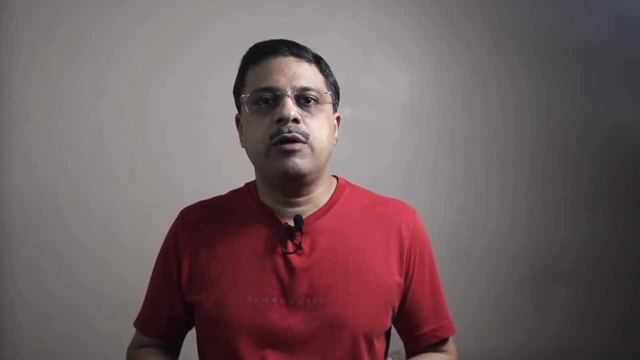 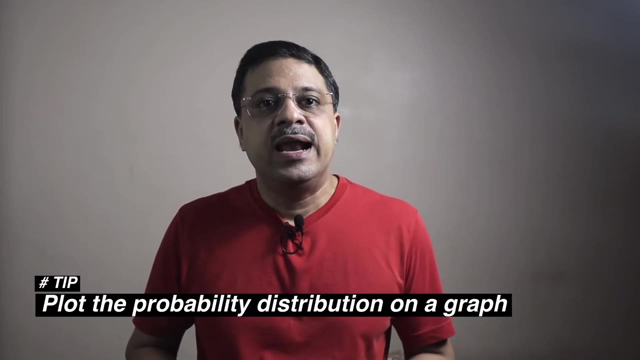 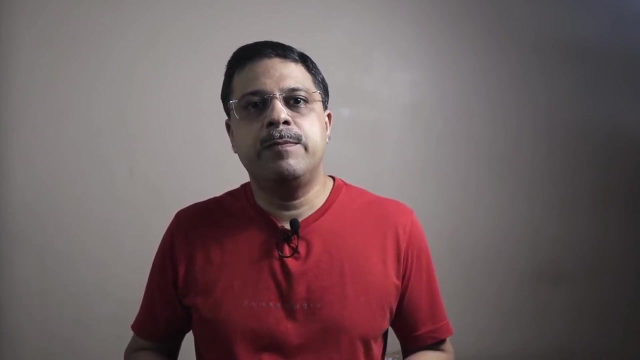 If this is representative of the population, then, using the formula of a probability, we would have a probability distribution for the population like: so: Here's a trick. Life becomes easier if you always plot it on a graph. If you plot the frequency distribution, you get a bar chart or something like a histogram, And if you plot the probability, 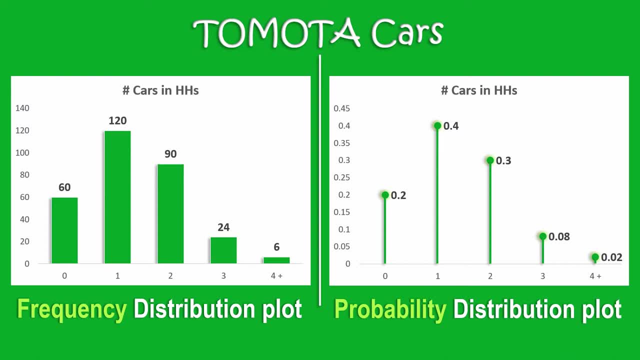 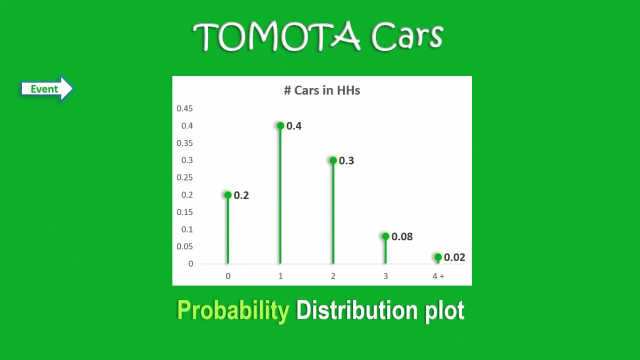 you get the probability distribution plot, or also called the probability mass function plot, or PMF plot for short. Hope you've noticed how different they both look. So here's an important tip. To plot a discrete probability distribution, you need to identify an event. 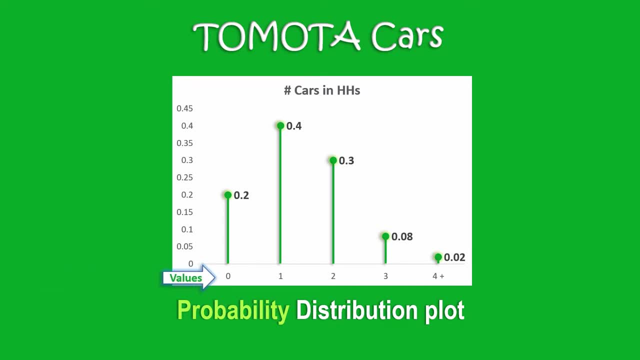 the possible values that the event can take, and the function that determines the relative probability that the discrete random variable is exactly equal to some value. For example, probability of owning over four cars is 0.02, or 2%. This function is called the probability mass. 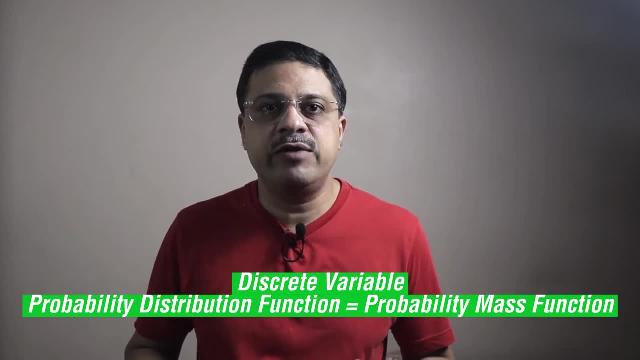 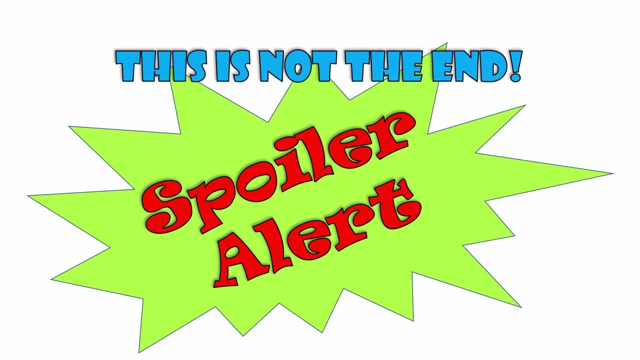 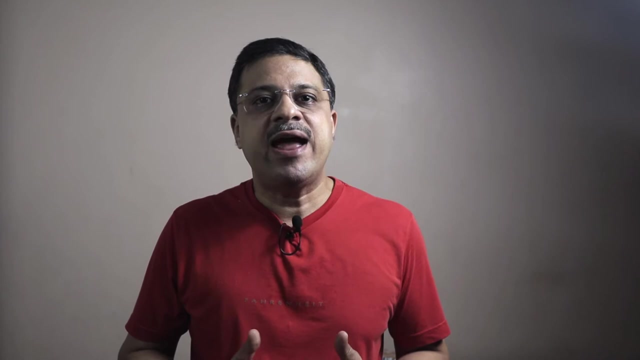 Note: probability distribution function for a discrete variable is same as a probability mass function. Spoiler alert: this is not the end. What we saw in the earlier two examples is called discrete probability distribution. It is discrete since the random variable, that is, the number of cars owned or the bucketed 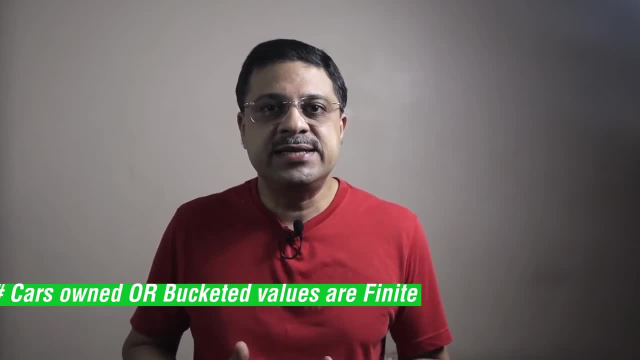 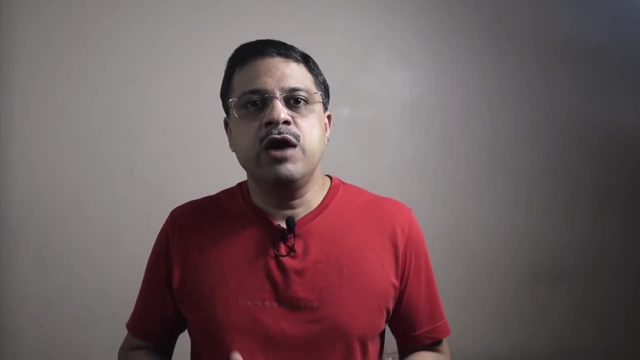 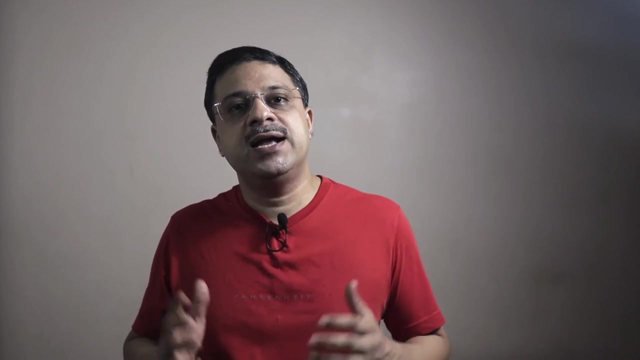 age groups take on finite values. This means that we can also have a continuous probability distribution that is based on continuous variables. If you have seen this video over here on basic statistics, you would know that a continuous variable is one that has continuous values. 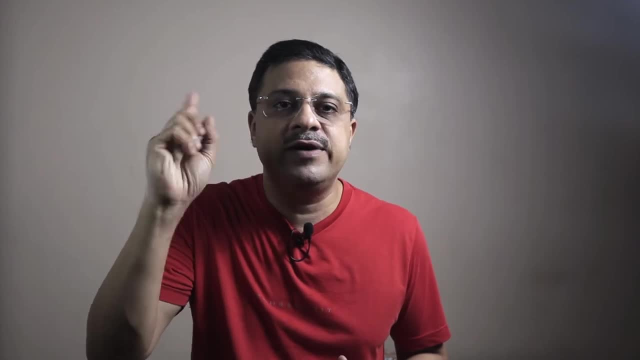 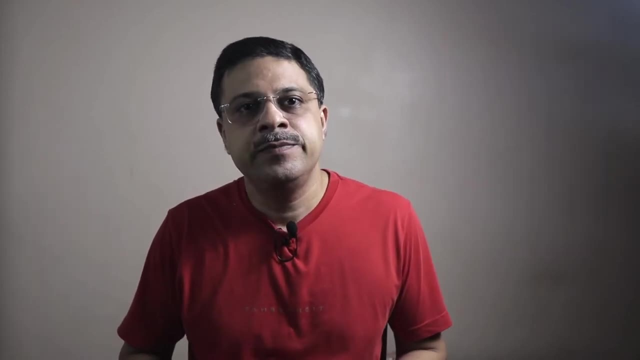 The link to this video is posted in the description below and in the info card somewhere above over here. Alright, let's move on ahead. We all have a set of tube lights or bulbs in our homes. These tube lights or bulbs come with a lifetime or a lifespan rating. 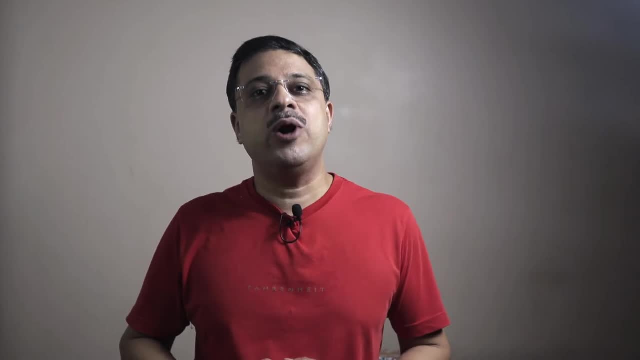 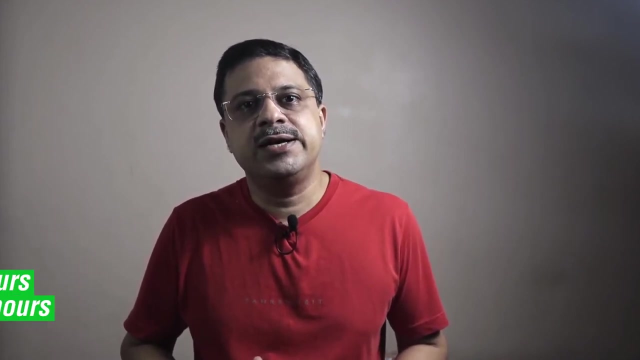 Bling lights, a manufacturer for electric bulbs, as part of quality control process, tests the various bulbs that get manufactured over a time period for their lifespans till they become non-functional. In one such test, the manufacturer found out that the few thousand bulbs tested lasted. 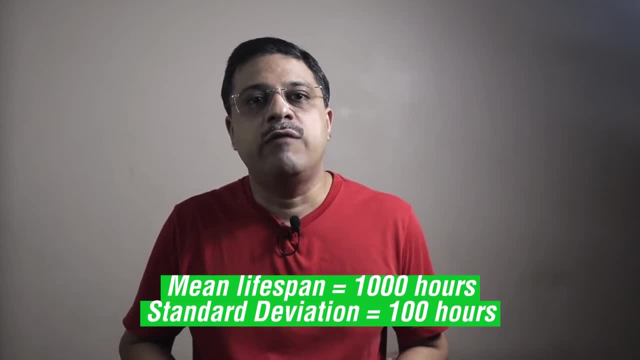 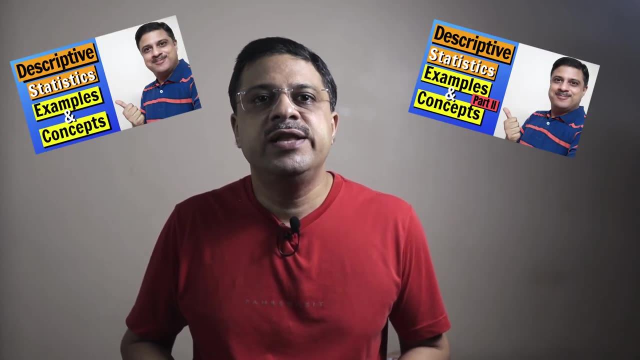 on an average for 1000 hours, with a standard deviation of 100 hours. To know more about mean and standard deviation, I would suggest that you watch these videos, for which the link is posted in the description below and the info cards posted above somewhere. 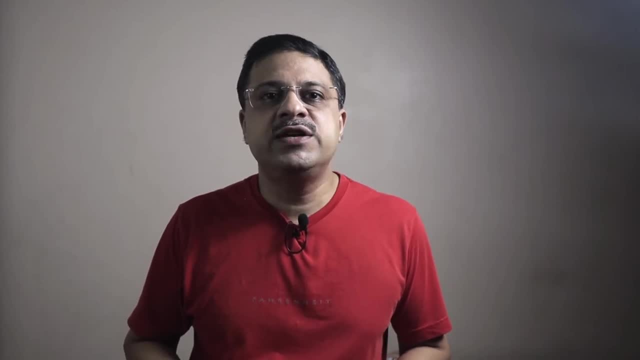 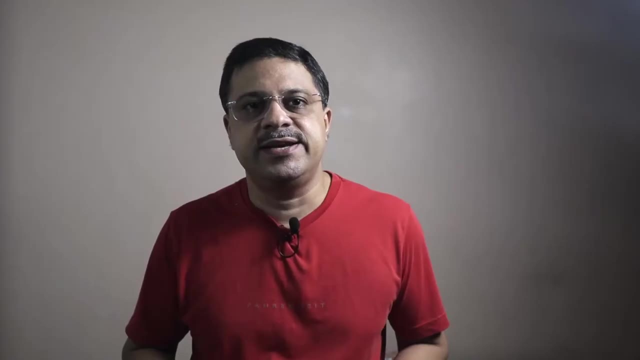 over here. For simplicity sake, let's take only a sample of 31 readings depicted in this table. The readings indicate the lifespan, hours of the 31 bulbs tested. If we observe the table carefully, we will notice that, unlike the earlier examples, the 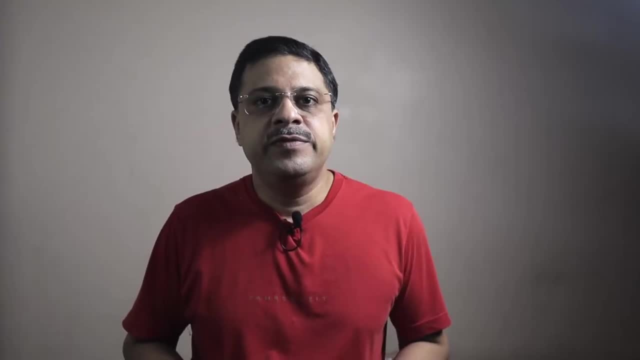 values here are in decimals as well. There would be several thousand bulbs- not part of this sample- that would have different set of infinite range of values for their lifespan. This indicates a continuous random variable. Let us look at two groups of thiscke value based on generalек probability distribution. 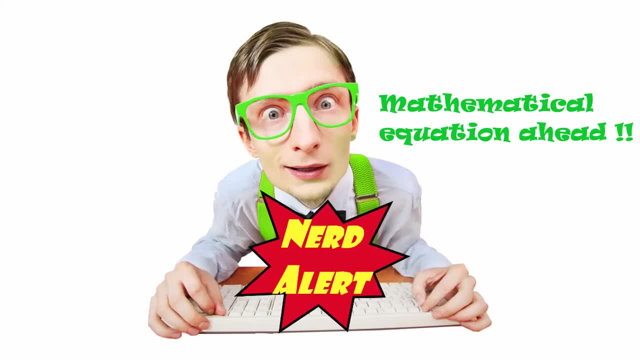 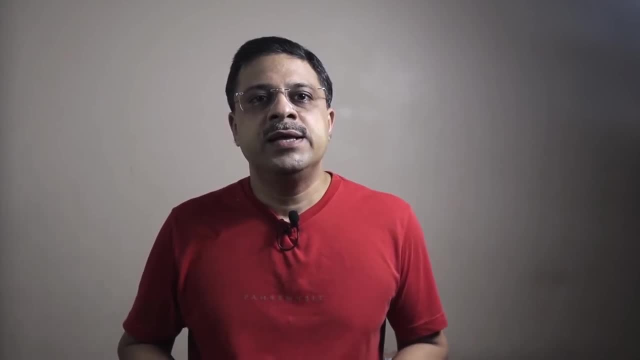 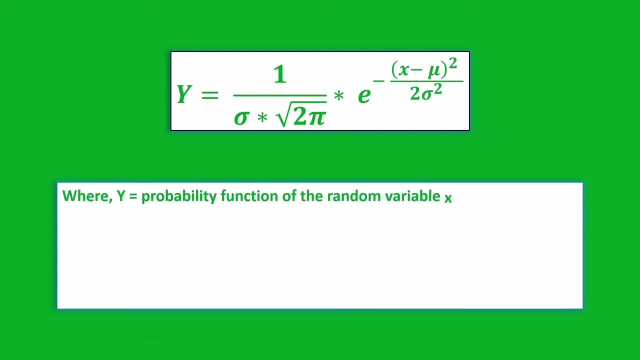 Before we move on ahead, a word of caution. The most used continuous probability function is the normal distribution function. This is depicted by the following formula, Where y is the probability function of the random variable, x. X is the normal random variable, in our case lifespan hr. 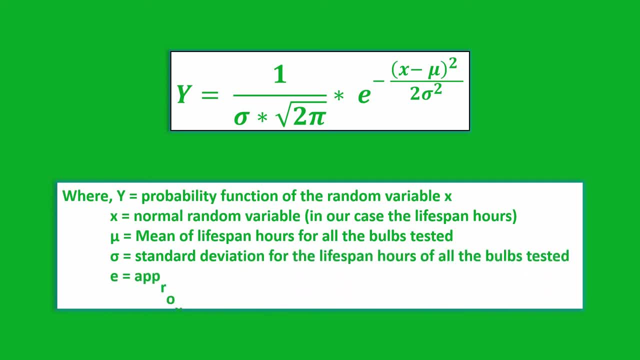 Meh is the mean of as lifespan hr. 8vxvx, 7i5-0.886,лат6.. kx2, x7,, 8,926.2readsxk$Oxx$ for all the bulbs tested. 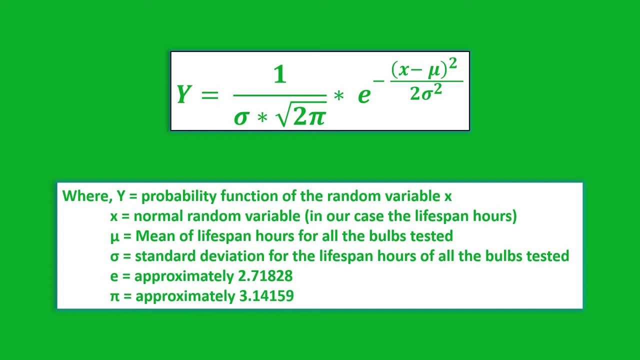 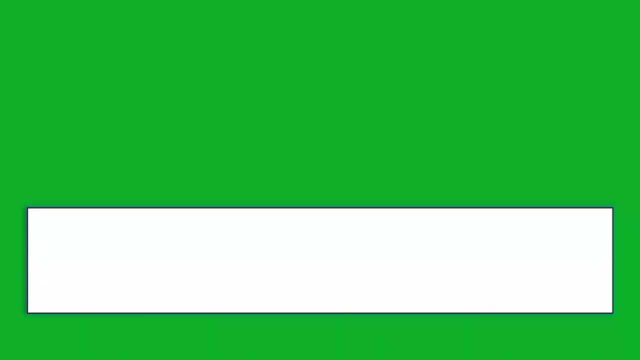 Sigma is a standard deviation for the lifespan hours of all the bulbs tested. E is approximately equal to 2.72.. Pi is approximately equal to 3.14.. Let's take one such value, that is, 1190, from the table and replace each of the values in this equation. 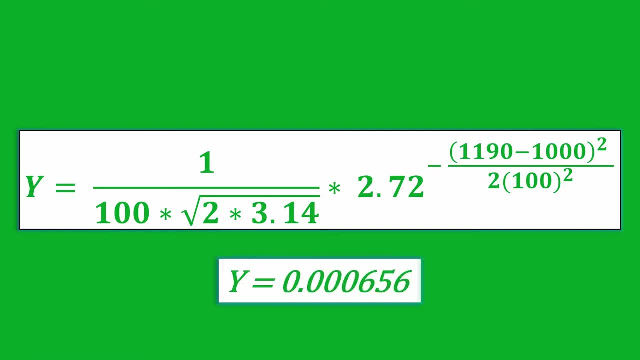 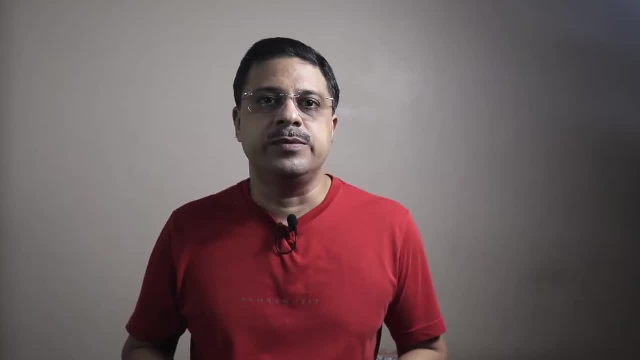 We get the probability, which works out to be 0.000656.. If we calculate the probabilities for the table, we get the following probability distribution And when we plot them, this is what we get. Looks scarily familiar right? Yes, this is the normal distribution. 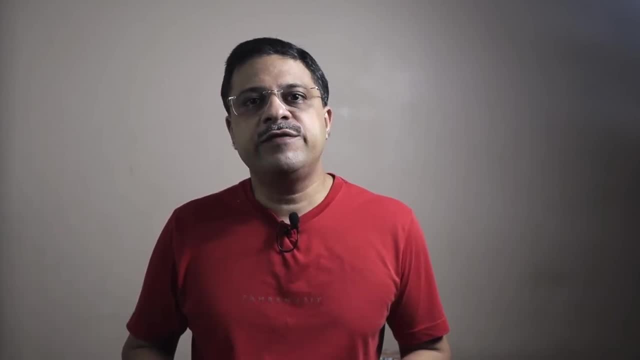 or the infamous bell-shaped curve. It is a part of the family of many other continuous probability distributions And no, this is not the only one. This was picked up only for the sake of simplicity. So to plot a continuous probability distribution, you need to identify one, an event. 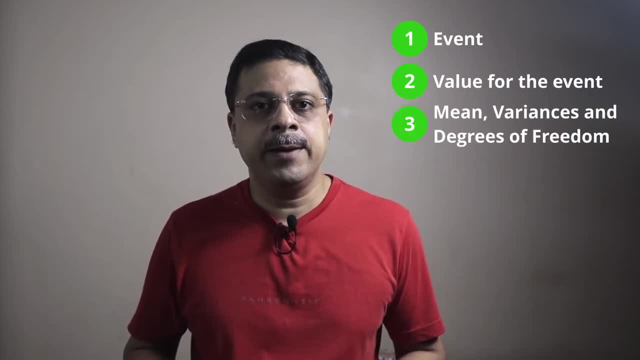 two possible values. the event can take three: the mean variances and, in some special types of distributions, a number called the degrees of freedom of the values for the event. Degrees of freedom in short refers to the number of values involved in the calculation. 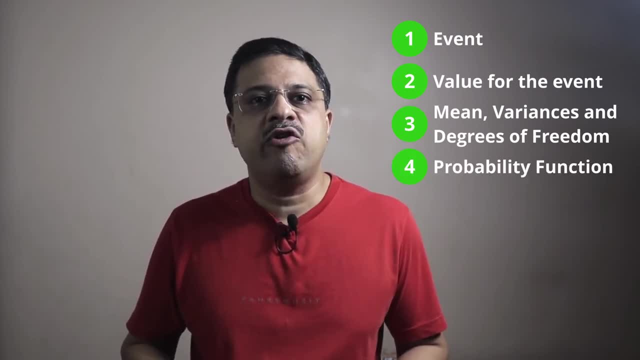 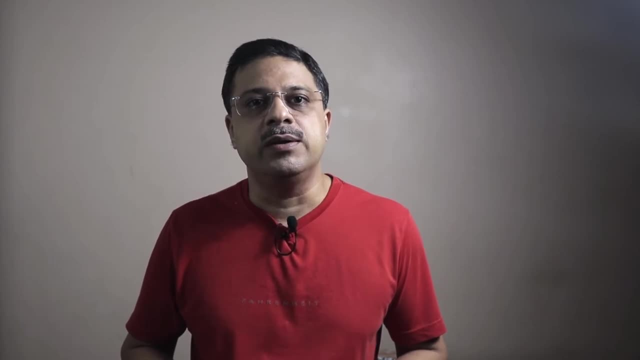 that have the freedom to vary, But we won't look at it right now. And the fourth one is the function that determines the probability distribution for the continuous random variable. This function is also called the probability distribution. It is also called as a probability density function. 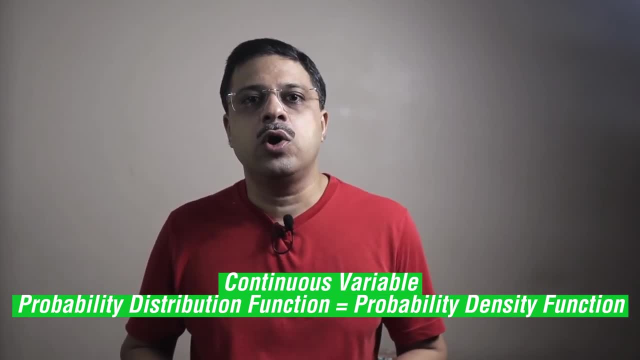 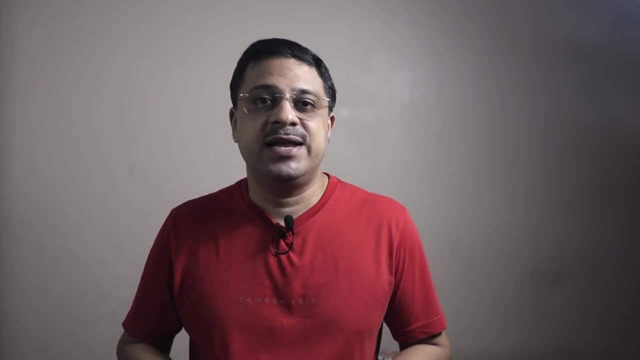 The plot of a continuous probability distribution is also called as a probability density function or the PDF plot. Don't mistake it with the PDF document. It has nothing to do with it. So there you go. It does not matter if the variable has a single value. 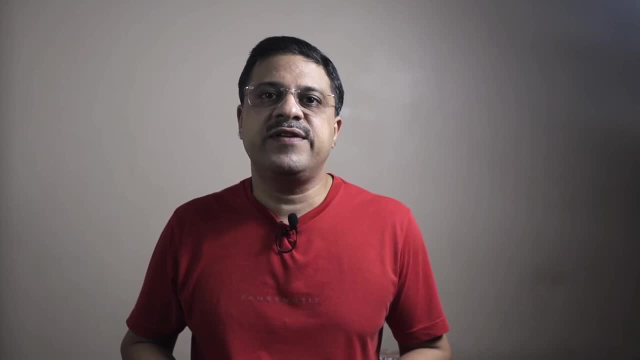 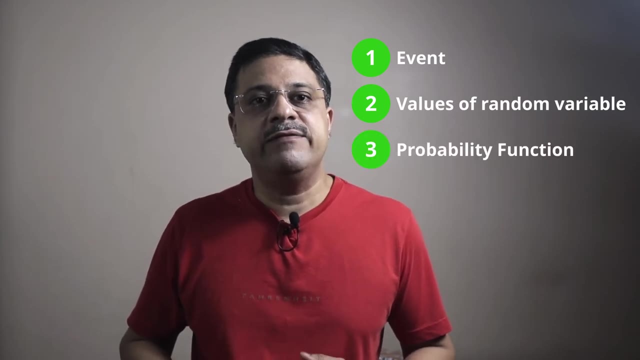 bucketed values or a range of values, as long as it satisfies the following three factors: that is, there is an event, there are possible values- a random variable for the event can take- and there are possible values- a random variable for the event can take. 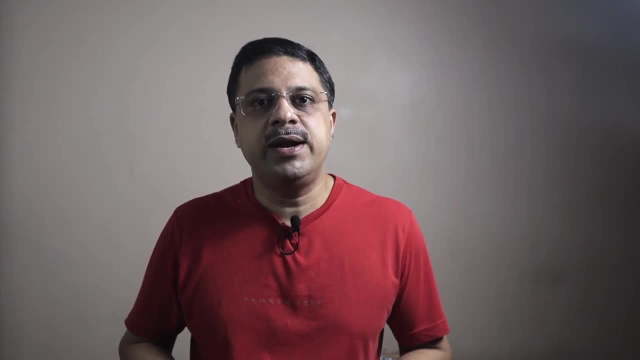 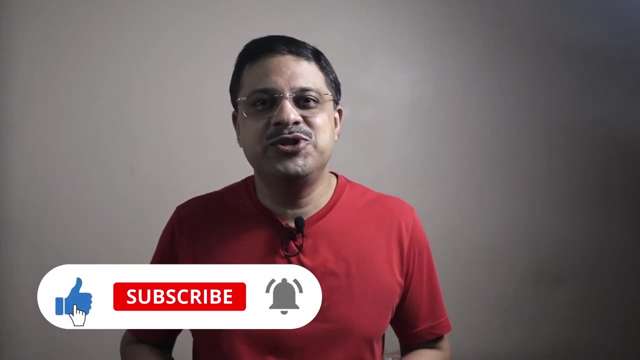 And a function to describe the probability distribution. you can always plot a probability distribution for almost anything. Simple, isn't it? So, now that you've become a super champ in plotting probability distribution from real-life scenarios, consider subscribing to this channel, and remember to click this bell. 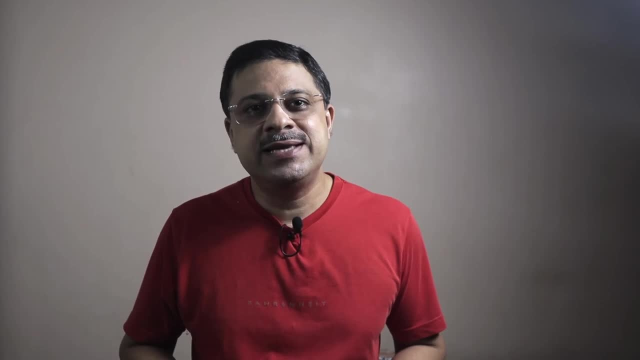 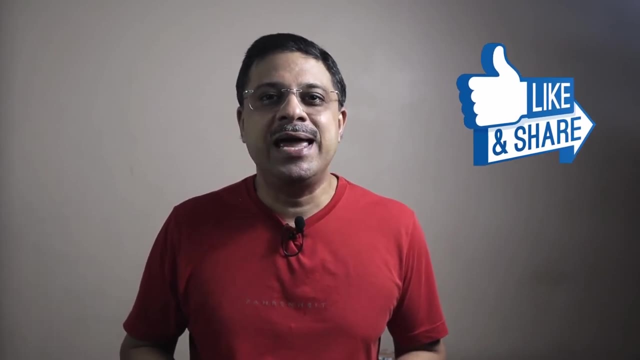 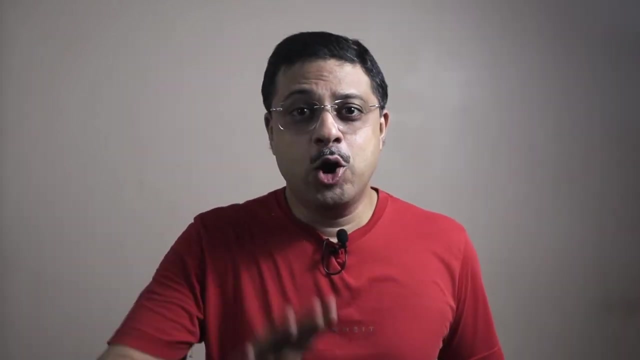 and not the probability curve. This way, you will not miss any videos that I upload. And, oh yes, please do like the video so that YouTube can promote this video to help like-minded people to update their understanding on probability distribution as well. How cool isn't it. 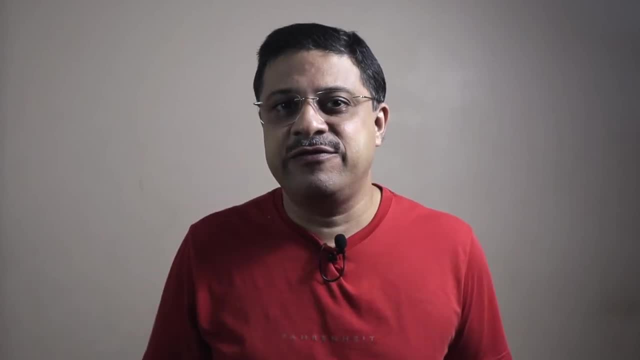 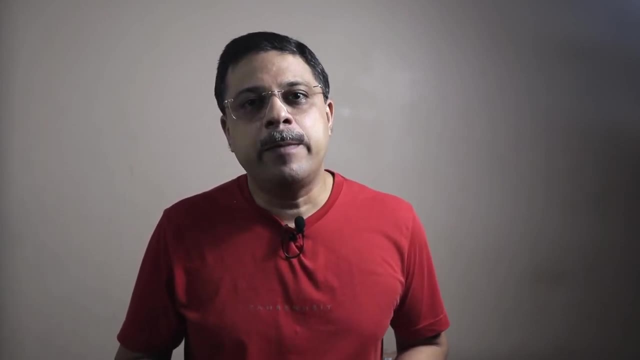 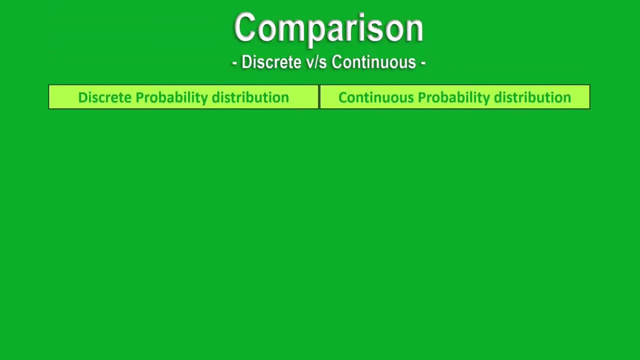 Oi, this is not over yet. There is still some interesting stuff to know about Now that we know about probability distribution. here is a quick comparison table of the properties of two types of probability distribution: As the name suggests, variable values for discrete probability distribution. 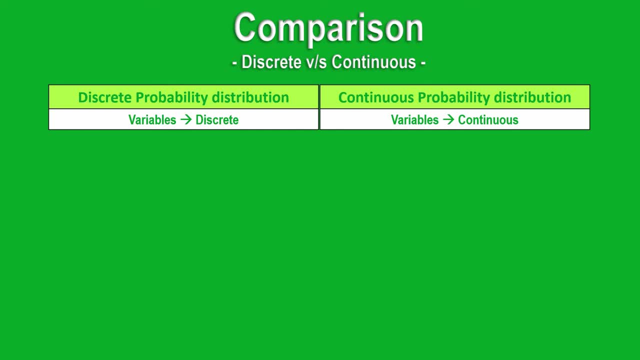 are discrete as against continuous. for continuous probability distribution, Discrete probability function is called the probability mass function, whilst continuous probability function is called the probability density function. For both distributions all probabilities are positive, Any event in the distribution, let's say scoring between any two values, A or B.